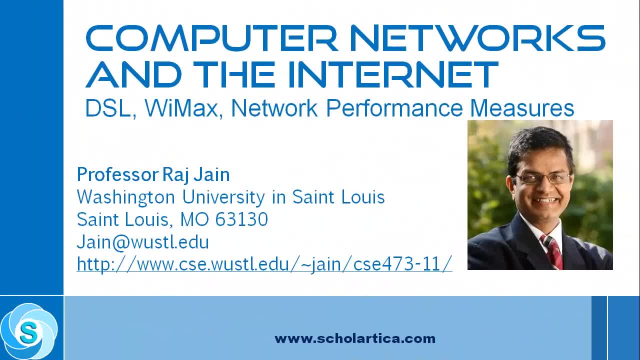 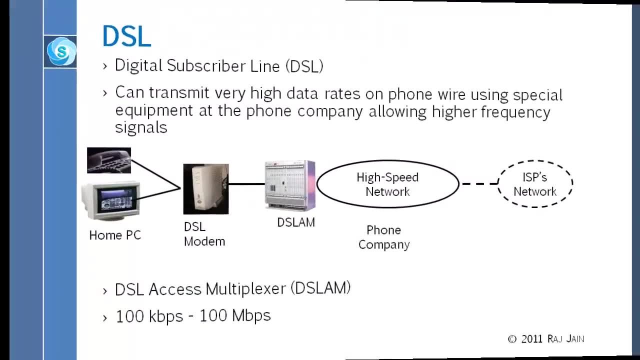 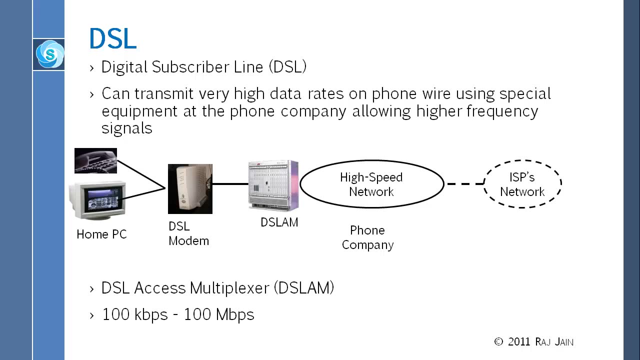 For BSL. one way to increase the speed is to get rid of, to make this line digital, the access line digital, And basically that's what the phone company did. You take the bits, actually you take the phone waves and you take the computer bits and combine them and 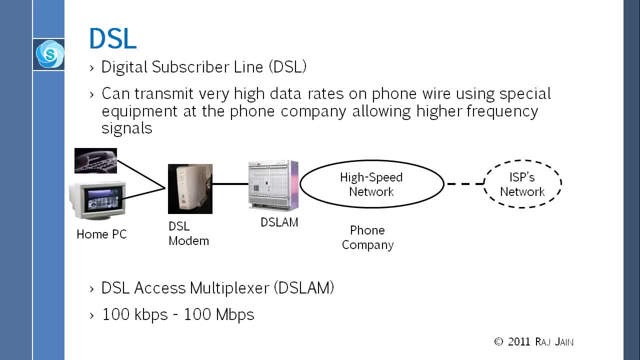 then send over and put a device here that can separate out the two. Basically these bits are coded at much higher frequencies. So this one is coded up to four kilohertz and this one is coded from you know higher frequency, like 20 kilohertz. 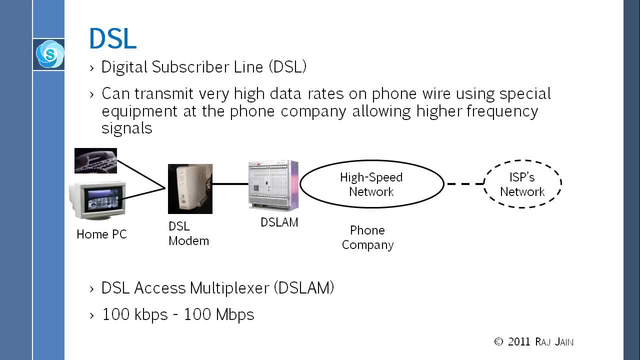 This one is coded to maybe one megahertz, So there is a frequency division multiplex in here And then here those frequencies are taken out and then you can get the bits out. So basically this is what is called BSL. BSL stands for Digital Subscriber Line, And this 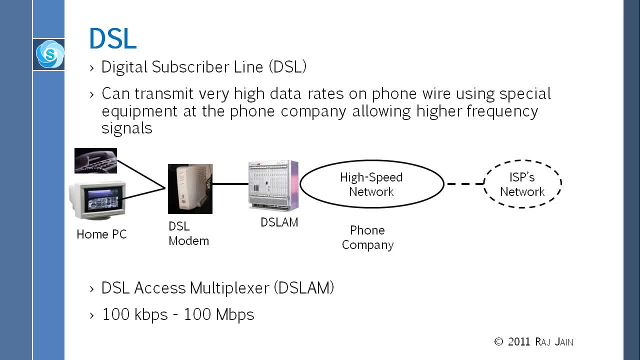 is your subscriber line. This is the line which goes from the phone company to the subscriber, which is you, your home. Once that becomes digital, that is called BSL, and now you are not limited to 56 kilobits. You can go up to as much as you want. I mean, I have a service for 18 megabits, which is 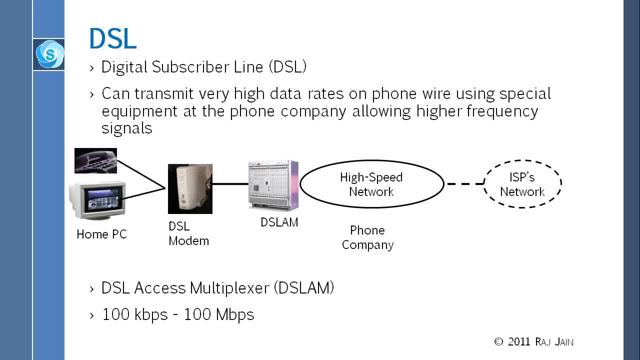 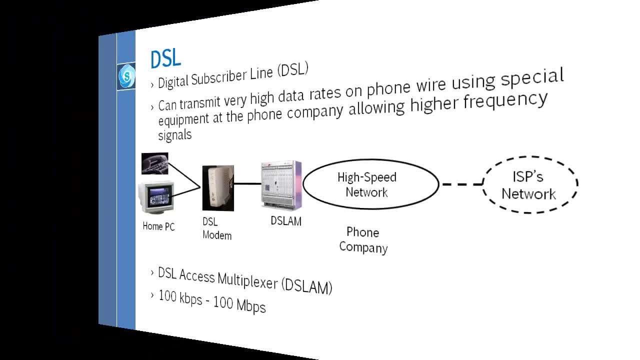 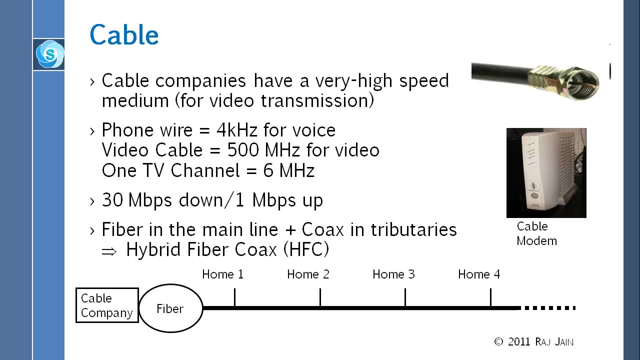 the highest available in St Louis, But, as I said, in Japan and Korea and other places you can get up to 100 megabits, And then this cable company can give you high speed too. Basically, what they do is they already have a cable which runs all through the streets and to your home, which is very 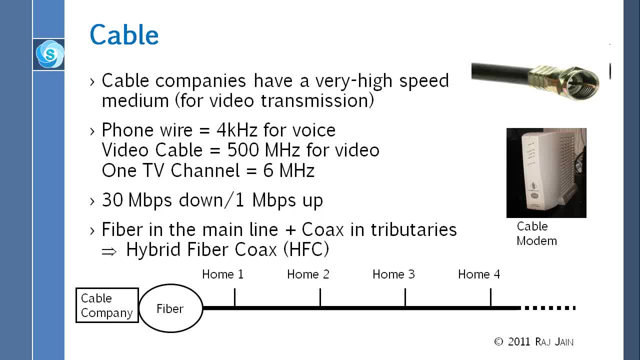 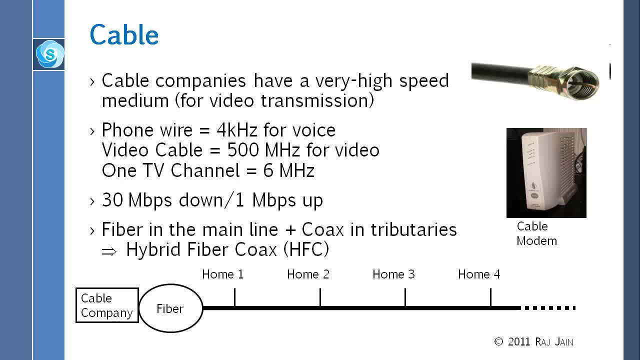 go up to 100 megabits And then you can go up to 100 megabits, And so you can see, this is the single channel that I mentioned in the 30 minutes, the single channel. So if you have one channel you need 6 megahertz If you're getting a 70 channel from the cable. 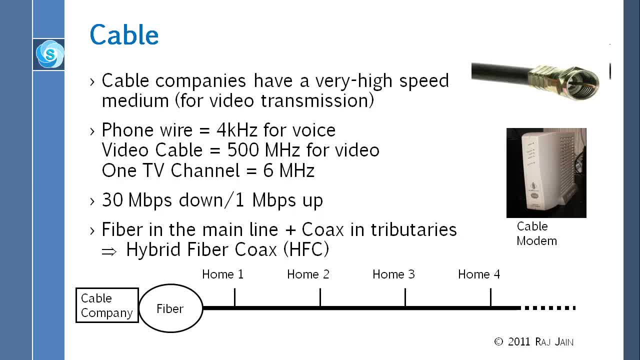 company. you have to multiply that by 70.. So 70 times 6,, so that many megahertz. But the video cable is good, It can take up to 500 megahertz, All right. And therefore, given that we use one channel for data, suppose we use one channel for data. 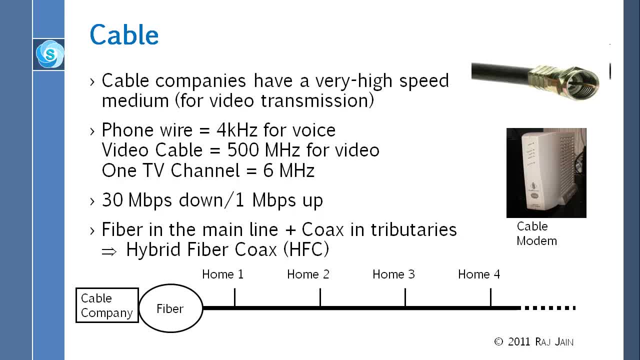 we do 5 bits per Hertz. if we do 5 bits per Hertz out of 6 megahertz, we can get 30 megabits. normally and the phone company and the cable companies offer service like this with 30 megabits down and 1 megabit up. 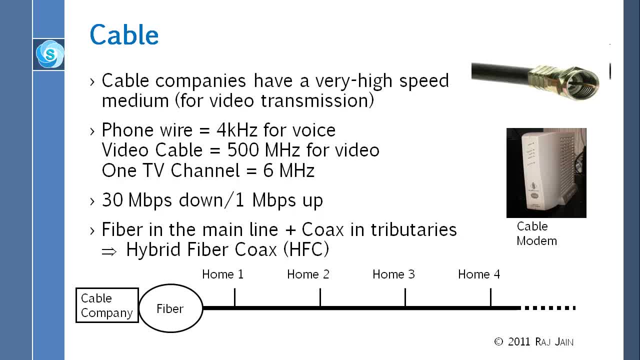 the up speed is always lower for many reasons that we learn about. if you learn when we learn about physically, and the down speed is 30, the up speed is 1. however, this all the way does not go. this cable does not go from your home to. 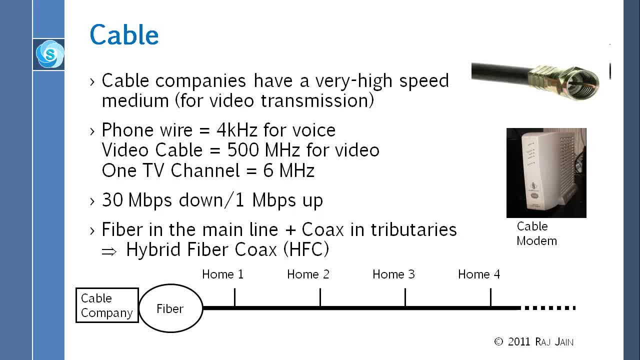 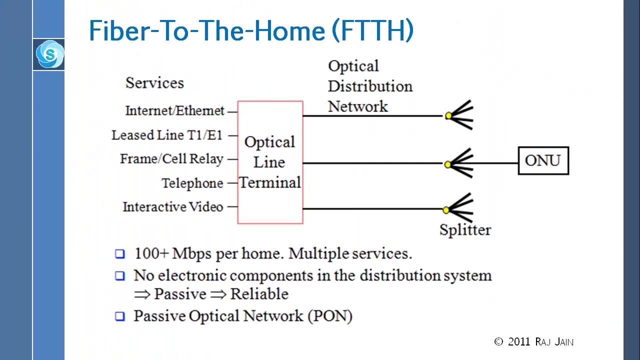 the cable company. what they do is they take it to some neighborhood and then they switch on to fiber and the fiber goes to the cable company. so that is why it is called hybrid fiber coax, HFC, the combination of fiber and the coax cable. in some places they have moved. 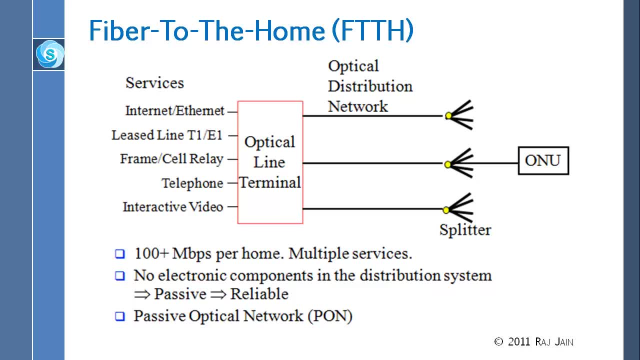 forward and they bring fiber to the home, and that is called FTP H. in the case of fiber to the home, what happens is that the whole things comes on a fiber and then at some places they have what we call the splitters, so the light that is. 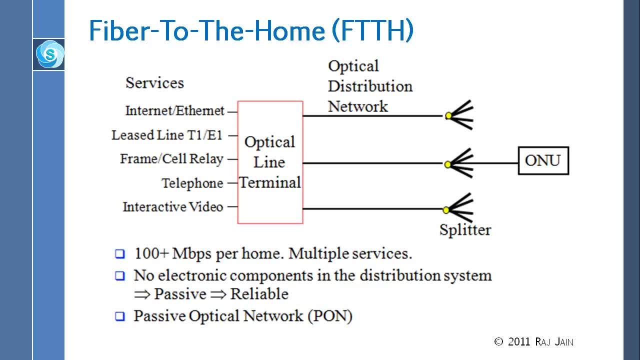 coming from here goes to all the fiber, better split, and goes to all the homes. so this is called optical line terminal and this is called optical network unit from UNOLT. so everything that you want to send to that become that you want to receive, such as Ethernet or d1, e1 at family or telephone or video, all. 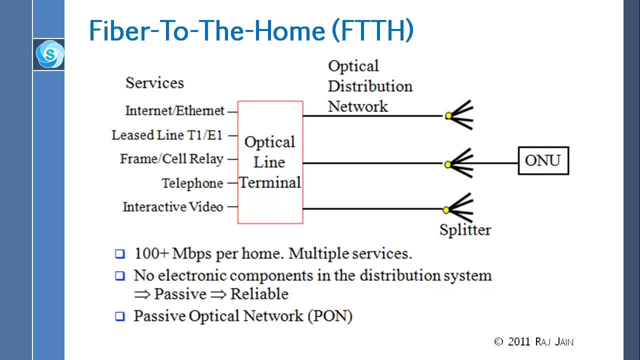 of that can be sent on the fiber. and since this is passive, this is goes every home, same thing goes to every home, and your O and U can select whatever is for your home and give it to you. And since this is passive, passive means there is no electrical power required. 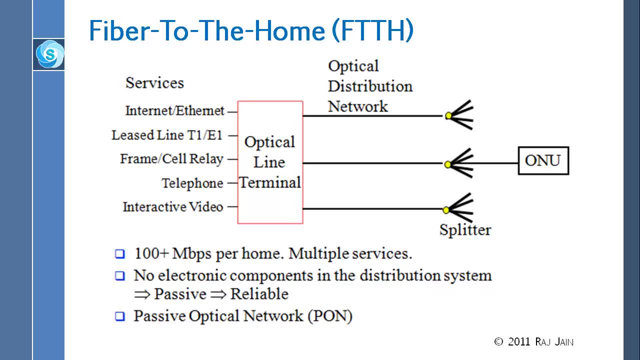 This is a simple splitter. There is no electrical power required. this is very reliable. they can put it on the curbs. If they needed a power there, then it can go bad and they have to send trucks to repair it. and all that. 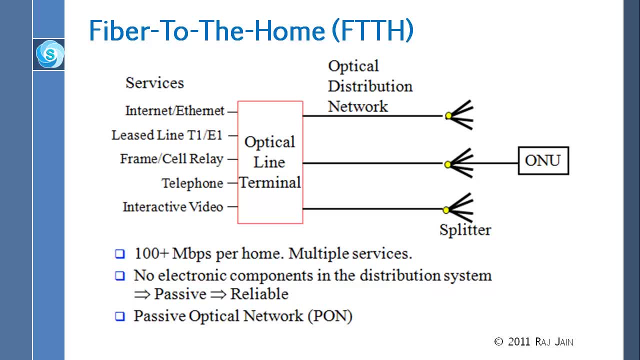 So that's why this is also called passive optical network PON, because of its reliability. So, like I said, I don't think we have in St Louis FTTH fiber to the home, but in some cities we do And again in other cities we do. 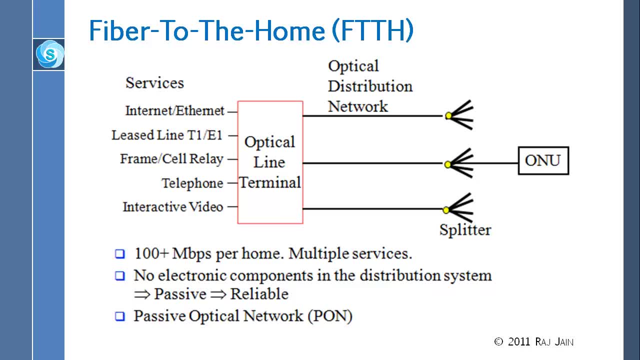 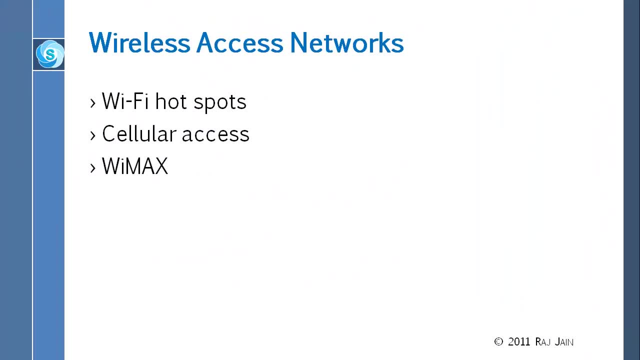 Okay. In other countries it's much more common, and again, the two countries that I keep telling you so many times is Japan and Korea. The next way to get to the network is wireless, and by wireless we have Wi-Fi hotspot cellular. 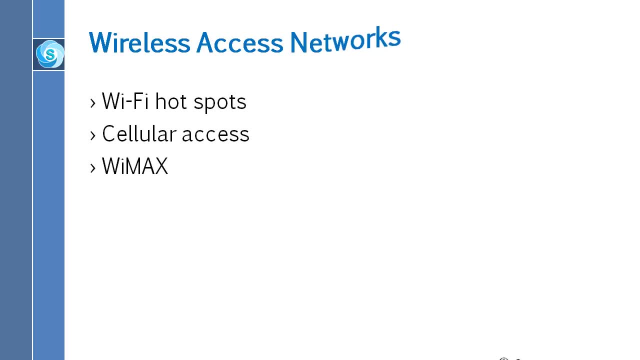 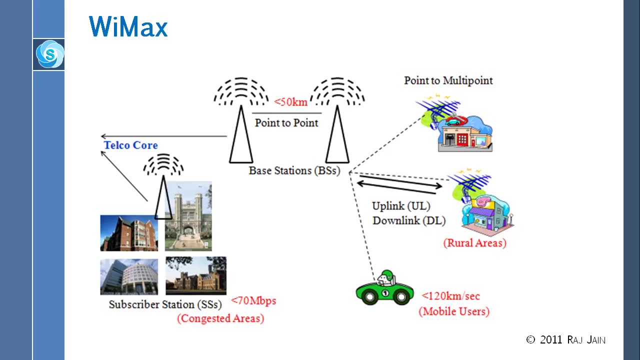 access telephone or WiMAX. So WiMAX actually is a new network that is just coming up and actually available in St Louis, And when you buy a computer nowadays it might even have a WiMAX- My computer, for example, the one that is in front of me here. 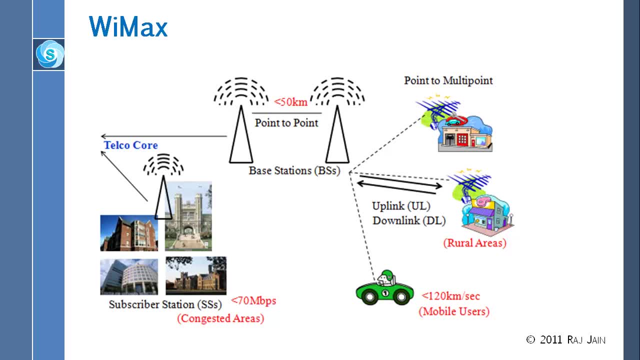 It has a WiMAX chip in it And Clearwire is offering this service here and if I were to get that service- it's like cellular service- I can go anywhere on the road, on the car, in the park, forest park, and I would be able. 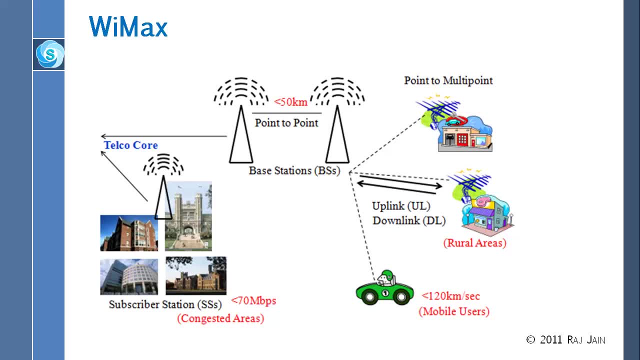 to get very high-speed access. Sometimes they call it 4G, which is a misnomer, because WiMAX is 3G, But it's not, It's 4G. They call it 4G because it's much faster than 3G- the current 3G. 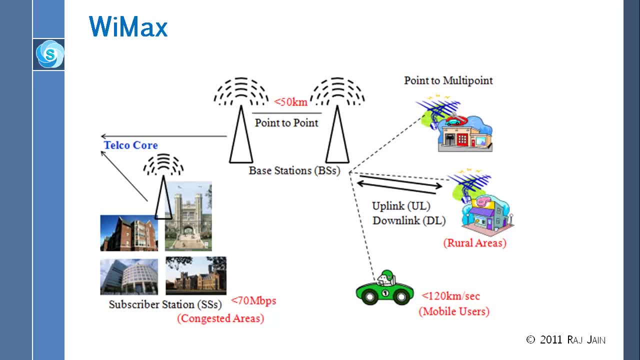 So I mean this is a names issue, but anyway. But the good thing about WiMAX is it goes as far as the cellular signal goes, but it goes at the speed at which Wi-Fi goes. The cellular signal is very, in terms of data rate is very low data rate right. 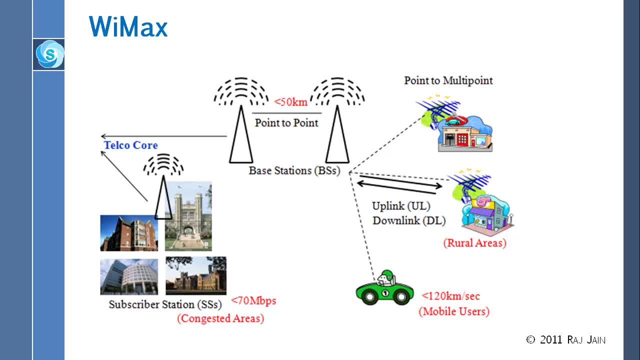 But WiMAX gives you very high data rate, like Wi-Fi. so it takes the best of Wi-Fi and the best of cellular. It takes the distance from the cellular, It takes the speed from Wi-Fi, So you can use it. You can basically, from one tower you can light up almost a city four or five kilometers. 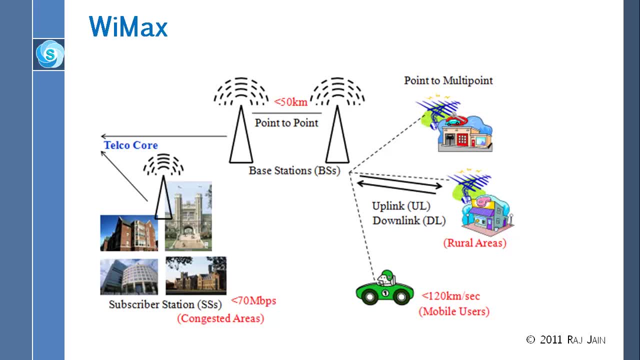 And you can even use it while moving, just like a cellular phone. That's all about the access. So we talked about the access, many different methods. We started with the WiMAX, We went to the modem, then we went to DSL, then we went to cable fiber and then the 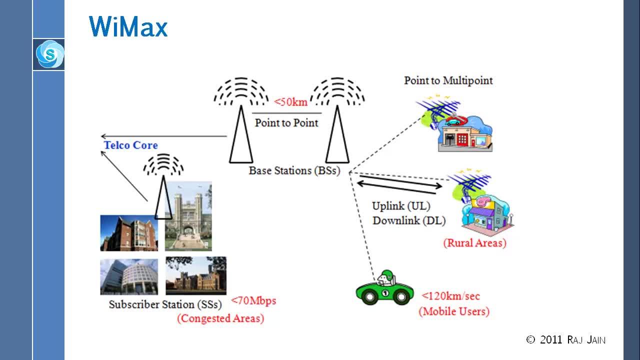 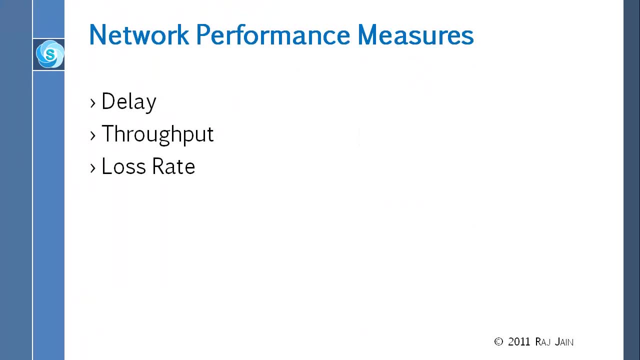 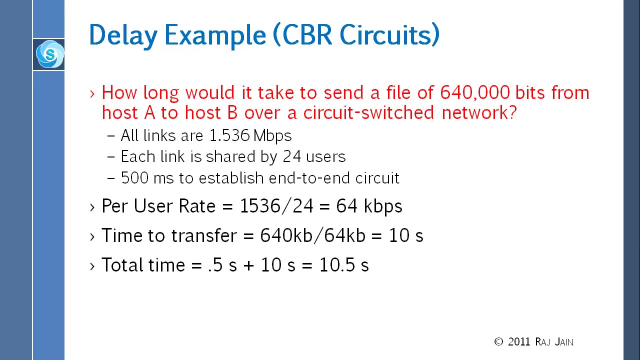 wireless. Those are all methods for access. So now we are back to networks and then we want to measure the performance of this. Then we move on to this. basically, three methods of measuring the performance: Delay. First thing we measure about the packet is: how long will it take? 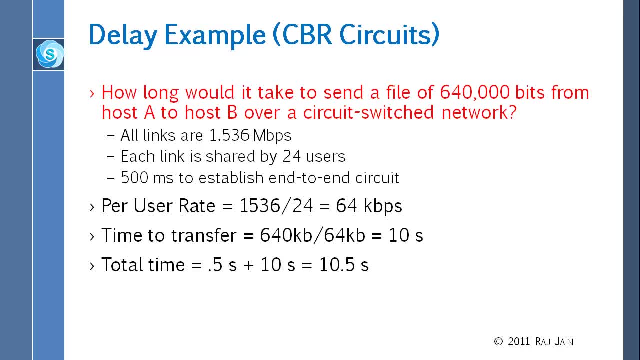 And then we measure the time, And then we measure the time, And so the delay consists of several parts. First is: how long will it take? So here's an example: So we want to send 640,000 bits over the circuit-switch networks and all the links are 1.536 megabits. 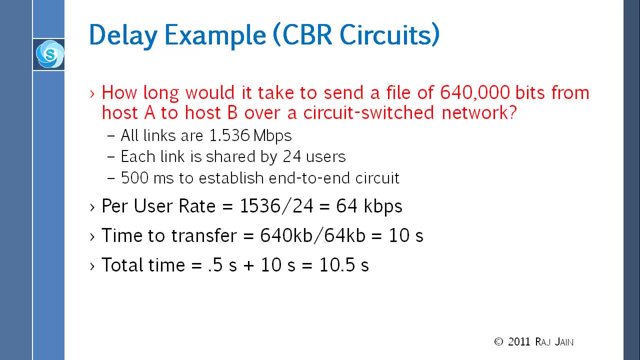 per second. Each link is shared by 24 users and 500 milliseconds to establish end-to-end circuit. So, since this is a circuit-switch network, just like a phone network, before you can send your first bit you have to set up the circuit. 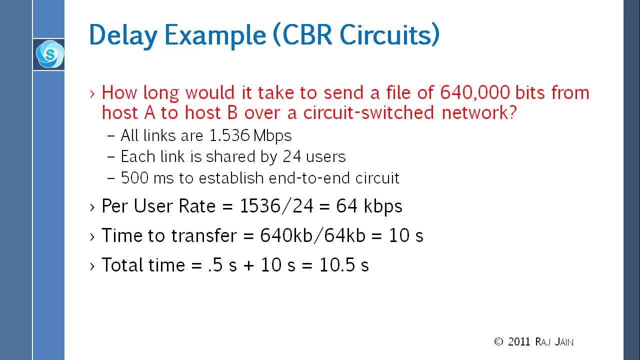 That takes 500 milliseconds. Once you have set up the circuit, then you can send either at 1: 24th of this rate, in which case you're just using 1: 24th- you're a single user- or, if you're a company, you 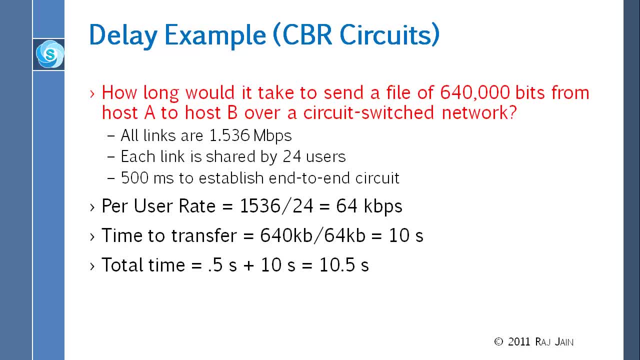 could get the whole line for yourself, For the company, and you can send at that rate. Basically the way phone line works is that the phone company right now takes 24 phone lines and puts them on one circuit That is called a T1 circuit. 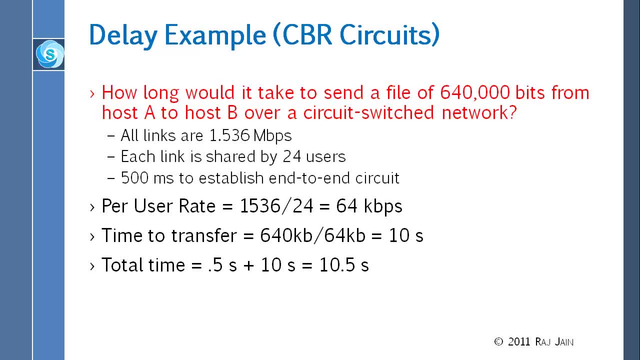 Okay, Each phone line is 64 kilobits. What happens is you. whatever you speak is designed. If you speak. it's digitized at 8 kilohertz. 8,000 samples per second. Each sample is 8-bit long. 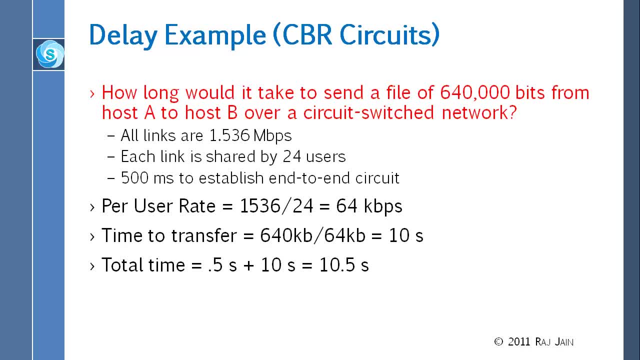 If you do 8 bits 8,000 times in a second, you get 64,000 bits per second. Okay, Now you take 24 users, so you multiply 64 by 24, you get 1536.. Okay. 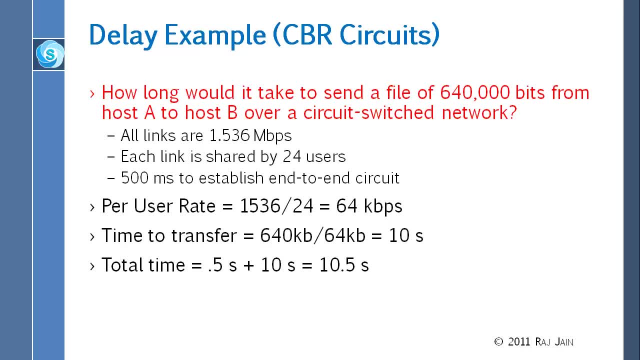 That is one circuit that the telephone company uses. That is called a T1 circuit. If you are a company, you could just ask for a T1 circuit. you get 24 lines and then you can use them for anything you want: for data, for voice or whatever. 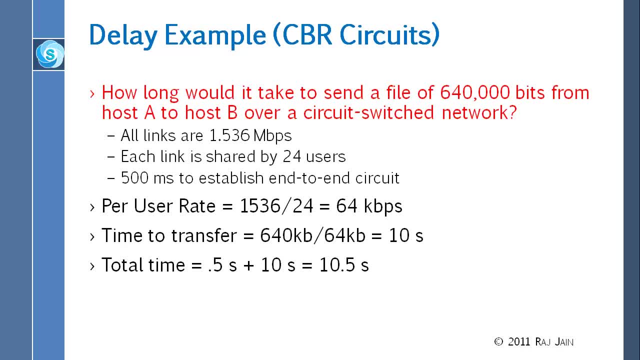 All right. So if you look on the wire, what you will see is 24 slots: First slot for the first user, second slot for the second user, third slot for the third user, fourth slot for the fourth user, 24 slots in a particular time and then cycle. 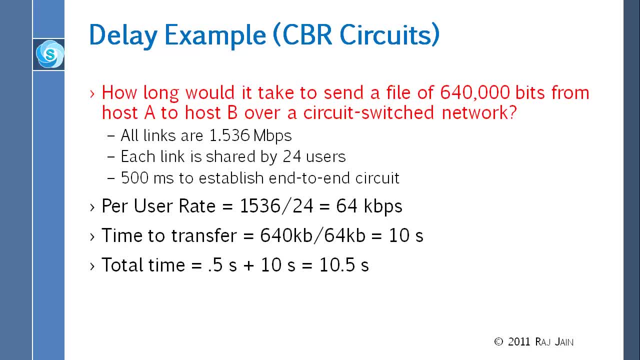 resumes again, Basically, then again 24 users. So all this happens at a certain rate. For example, in this example we are talking about one user. So one user will get only 64 kilobit and therefore to transmit 64, 640 kilobit it. 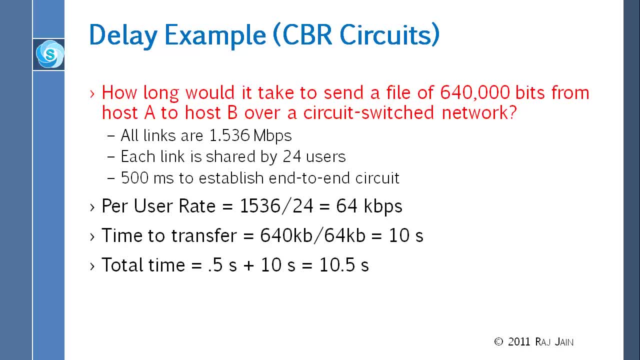 will take 10 seconds. If it was that, it was a WashU and WashU probably has many T1 links. Right, We cannot live with just 24 phone lines. We need probably 200,, 24,, 130 phone lines or something like that. 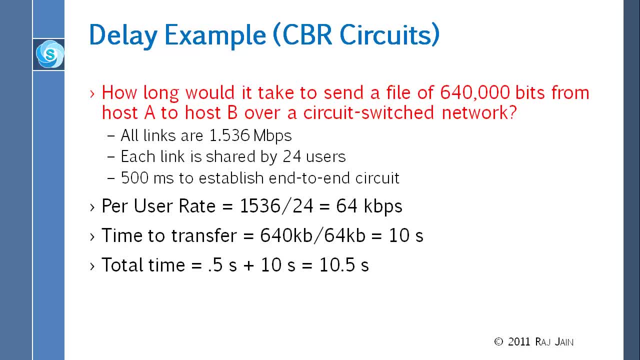 So we have many T1 circuits And so whatever rate you have, you just do that, Okay. And the second thing is that these rates somehow will come into. For example, for us who work on these things. we remember 1.536 T1, T3 is 45 megabits, T4. 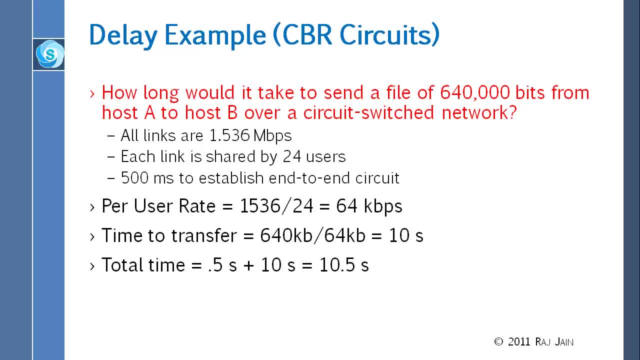 is something- All those numbers we remember because we work on them so often, right, But it will be clear whenever the problem is given to you as to what you have. Okay, So now it will take 10 seconds to send that many bits, but it will take .5 seconds to. 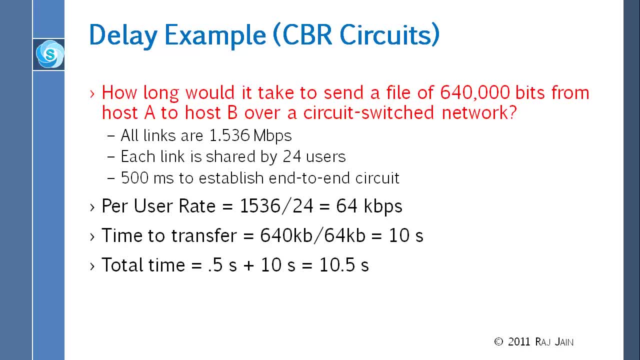 set up the connection, so the total time for that file would be 10.5 seconds. On a circuit-switch network, you need to set up the circuit and then send the bits. On a packet-switch network, you don't need to set up the circuit, you can start sending. 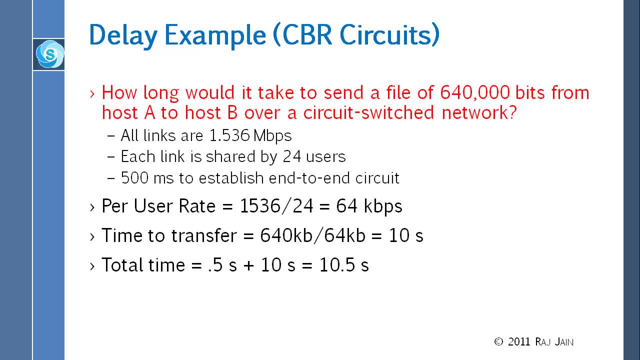 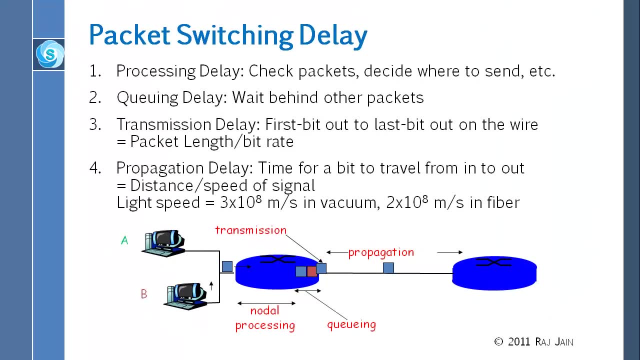 the bits, but you have to packetize it, so there is an overhead per packet. So let's talk about packet switching On the packet switching. first. you have to collect the bits as they're coming in, make a packet, add the header, put them in the queue. so there is a queuing delay as well. 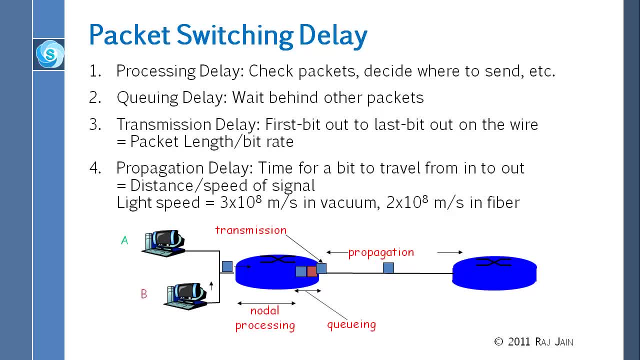 So there is a queuing delay, because you will be first, there is a processing delay, then there is a queuing delay, Okay, Then there is a transmission delay and there is a propagation delay. So what is transmission? what is propagation? 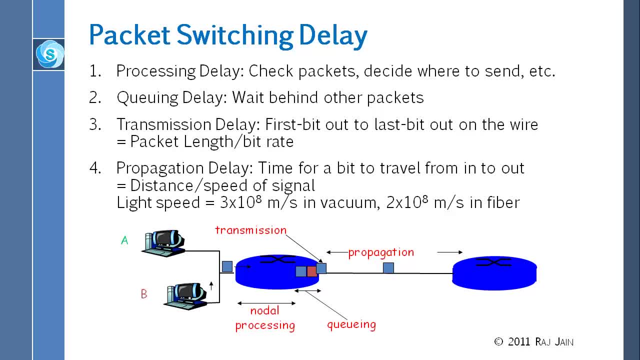 Transmission is for the bits to get on the wire. You see, when you have packet which is so big, first bit gets on the wire, then the second bit gets on the wire and the third bit gets on the wire. So let's say your packet is 512 bits, all 512 bits get on the wire and then they move. 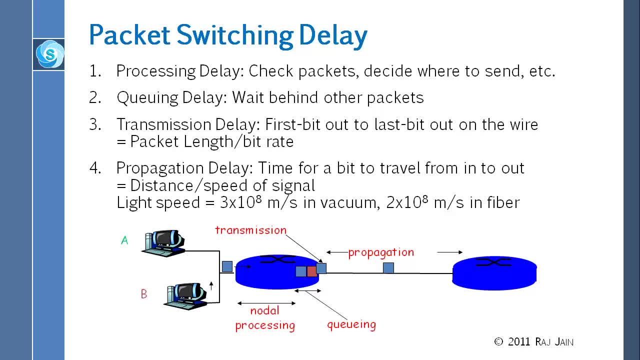 slowly to the destination Right. So that is the propagation delay. Propagation delay is the delay to go on the wire and to move on the wire Right, And the transmission delay is the delay to get on the wire. Understand the difference. 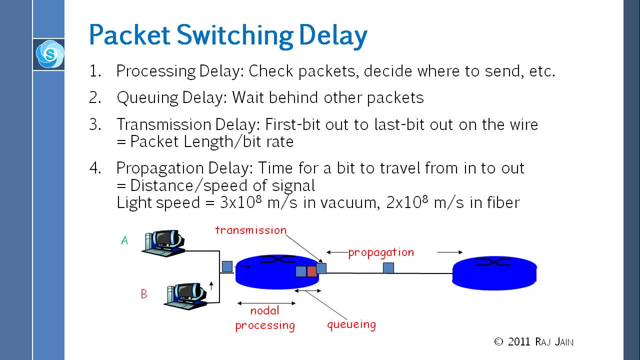 First the bits have to leave the computer and get on the wire. That is transmission. Once they're on the wire, depending upon the length of the wire they have to propagate. If the wire is, you know, 2,000 kilometers, they will land on the wire. 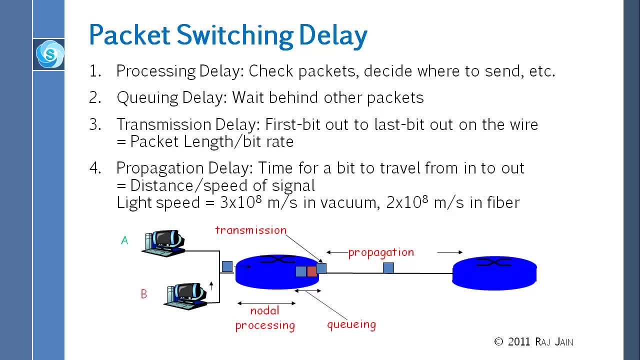 Okay, If it's 2,000 kilometers, there will be a lot of propagation delay, But the transmission delay will still be the same. Transmission delay simply depends upon how many bits per second you're transmitting and how many bits you have. 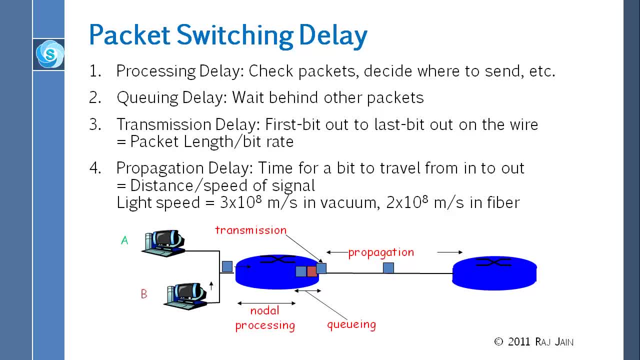 Right. The propagation delay depends upon the distance. So that depends upon the distance and the speed of the signal. And the speed of the signal is the speed of the light, which is 3 times 10 to the 8 meters per second. 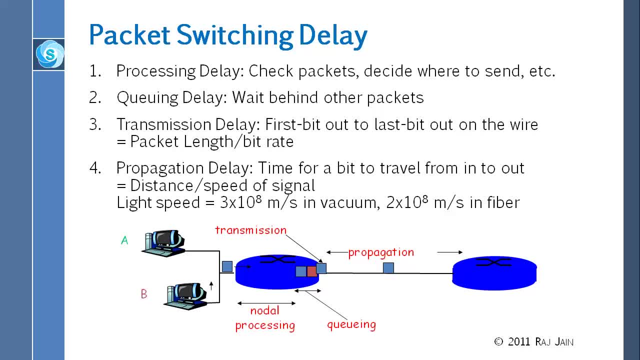 That is also the speed of electricity, Right? Yes, What is the speed of electricity? Well, actually, the speed of the signal changes on different things. So the speed of the light in VEC1 is 3 times 10 to the 8 meters per second. but if you're 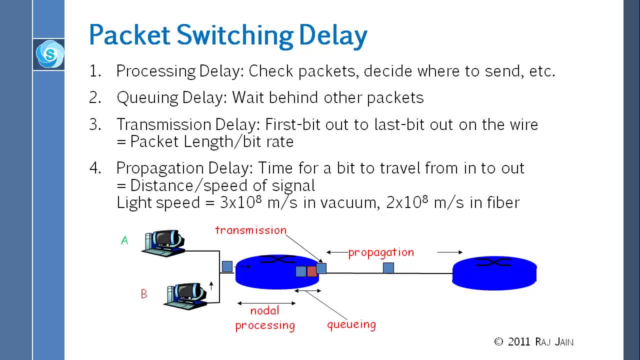 sending it on the fiber it is only 2 times 10 to the 8 meters per second. So you could have lines which are very long, You could have lines which are very short. You just have to know that. you know there are two distances. 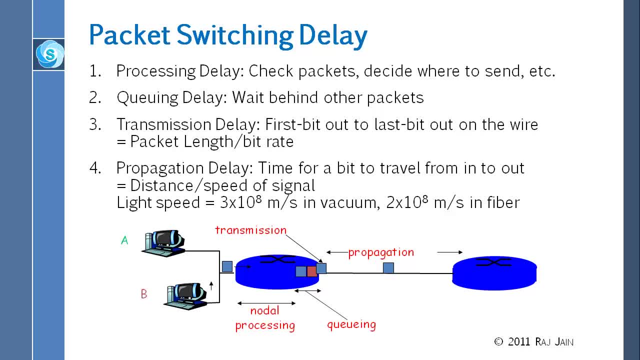 One is the distance to get on the wire, and the second is: you know so. the second is for the bits to reach the destination. There's no problem, Okay, So, all right. so we have to consider four delays: Processing delay, which is basically inside the computer. 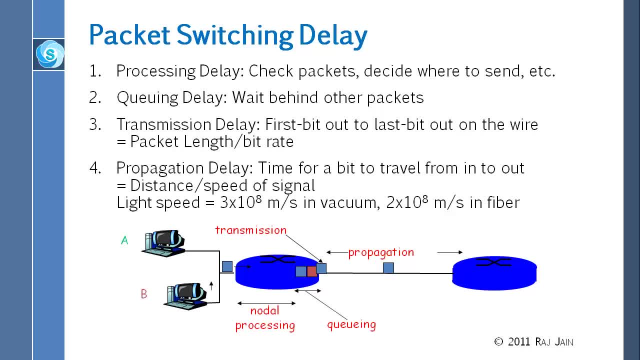 There you have to check out everything, make the packets and check the CRC and check that there is no error, nothing like that. Then you have to put them behind other packets. There might be a QN delay. Then there's the transmission delay and then there's the propagation delay. 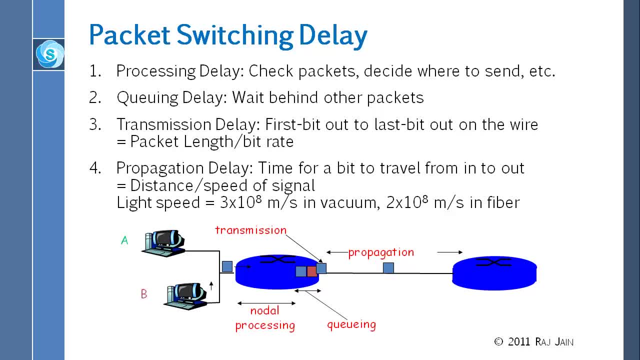 Okay, That's shown here. First, there is something that you need inside the computer. Okay, Once you get inside the computer, then you have to stand in the queue. Once you get your turn, then you have to get onto the wire and then, once you get on the 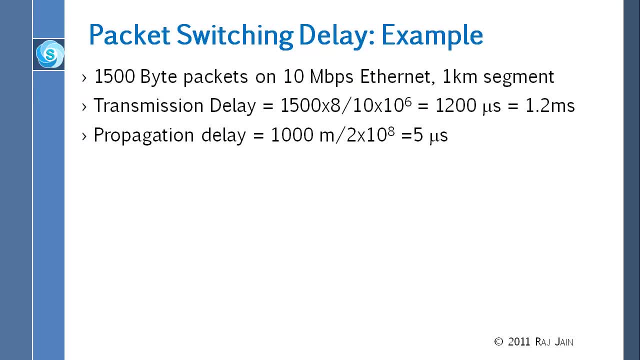 wire you propagate. So here is an example: You want to send 1,500 bytes on 10 megabit per second Ethernet and the length is 1 kilometer. So first of all, transmission is depends upon the packet size. 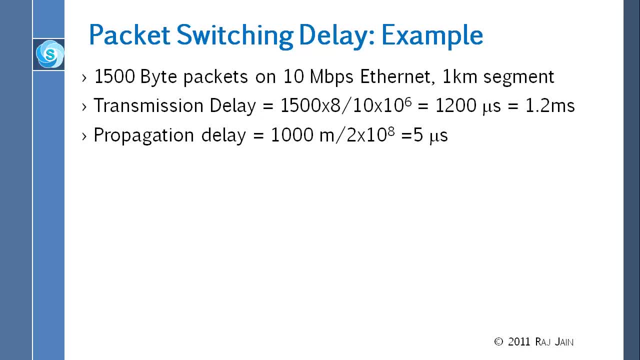 Because you want to get onto the wire. what is the speed they can get on? 10 megabits, And how long is the packet? 1,500 bytes. So how long will it take for the 1,500 bytes to get out of the computer at 10 megabits? 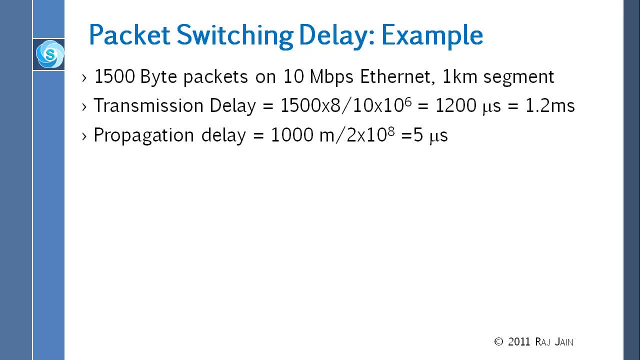 It will take 1,500 times 8.. Why 8? Bits per byte. 10 divided by 10 mega, 10 times 10 raised to 6.. That gives you 1,200 microseconds or 1.2 milliseconds. 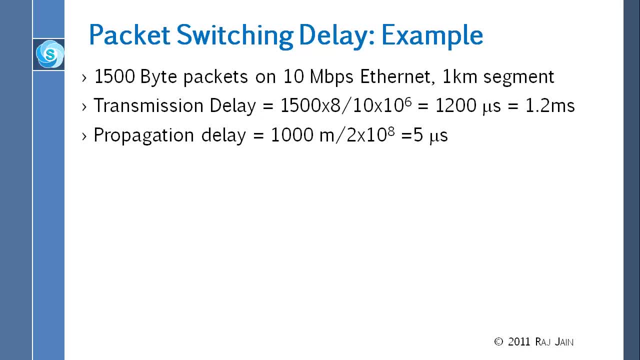 This is just the time that a packet takes to get out of the computer. get on the wire, Then the bits will travel to the other end, which is 1 kilometer away. And how long will it take for 1 kilometer? 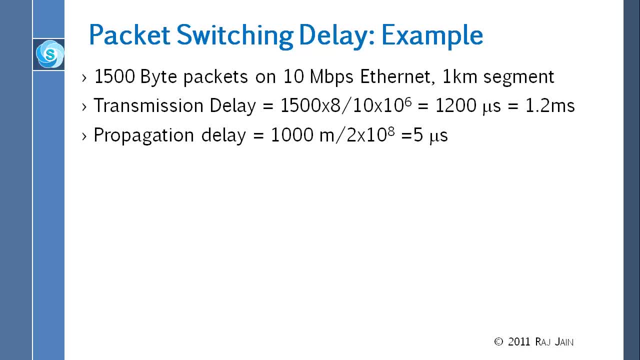 Since they're going on the fiber, we use the speed of 2 times 10, raised to 8.. And this is 1,000 meters. It takes 5 microseconds, All right. So it will take 1.2 milliseconds for the transmission delay and 5 microseconds for the propagation delay. 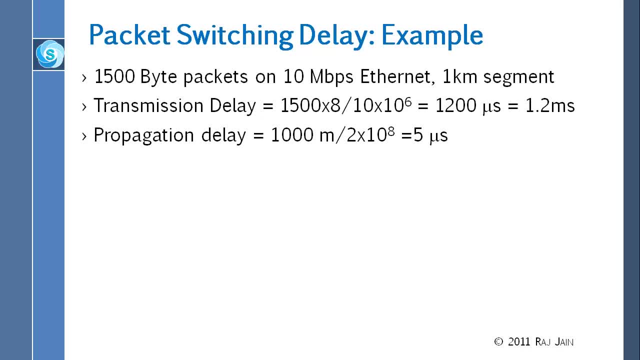 So that is the total delay. Actually, one delay which we have not calculated here is the queuing delay. It turns out as you can see here in this example, the propagation delay is generally small. What is large is the queuing delay, which is not large. 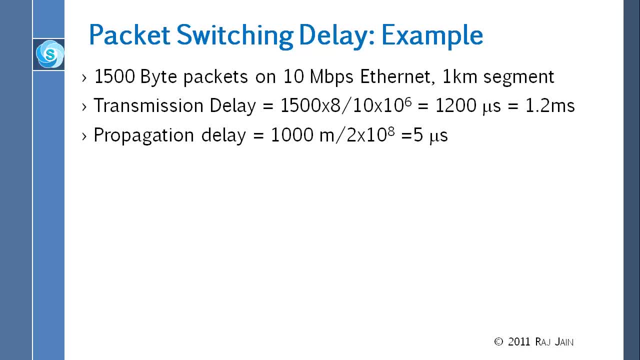 So that is the total delay. This is the queuing delay, which is not shown here. Queuing delay could be very large. It could be waiting inside the queue, Particularly in the router, where lots of people are sending the packets and then they stand in the queue to get out of the router. 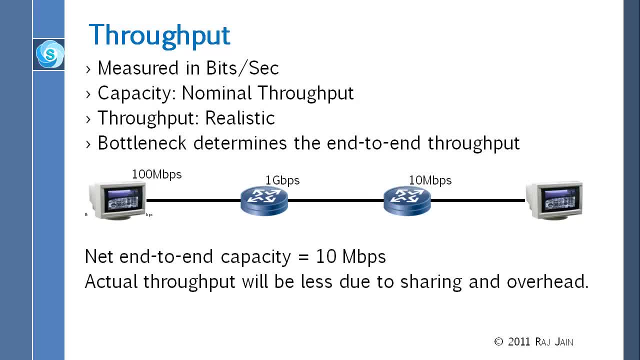 All right, so that finishes the delay part. So the key lesson is that if it is circuit switched, you have two delays. What are those two delays? Circuit setup and then the transmission, Basically the propagation, or whatever you want to call it. 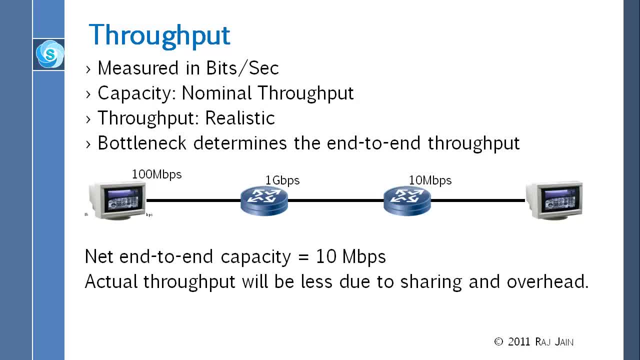 Propagation delay. yeah, If it is packet switched, then there are four delays: First is the preparation time, Second is the queuing delay, Third is the transmission And fourth is the propagation. Okay, So the propagation depends upon the distance and the speed of the light. 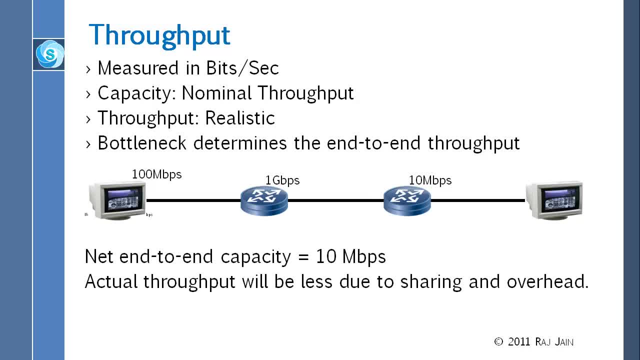 It does not depend upon whether you are going at 10 megabits or 100 megabits. You are still going 2 times 10 raised to 8.. By the way, that number 2 times 10 raised to 8, we all remember how. 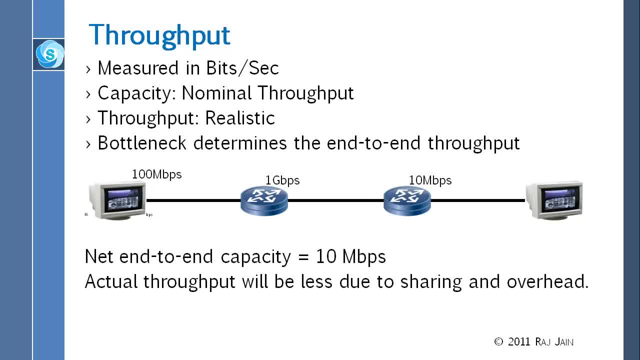 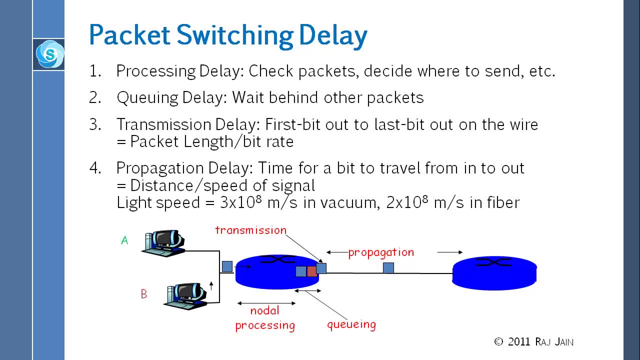 That number of speed of light. there are two ways to remember it. One is that we remember that it is 3 times 10, raised to 8.. That's kind of difficult to remember, but if you just remember 300 meters per microsecond. 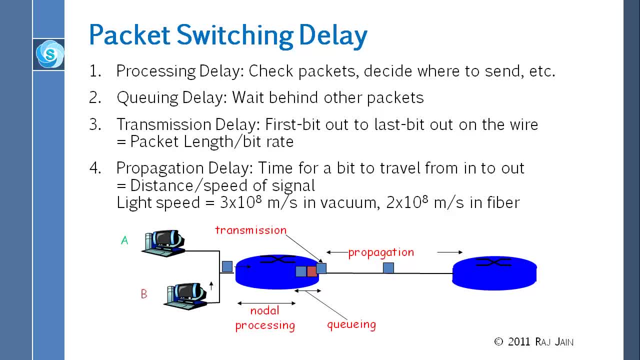 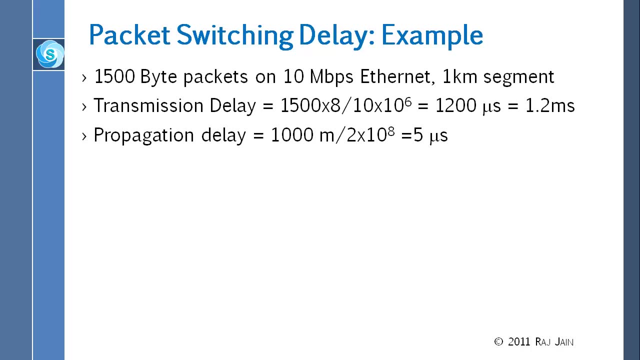 That's much easier to remember Because then the power goes away. 300 meters per microsecond. Second way we remember is: actually this is fiber thing which we use more often is just this number In our daily calculations. we know that it takes 5 microseconds per kilometer. 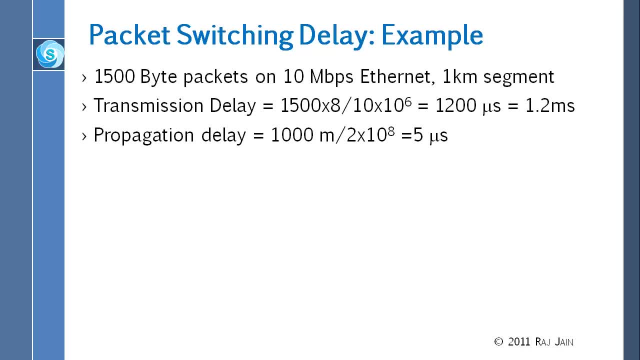 Period. That's it 5 microseconds per kilometer. So if somebody says that I have a link which is 20 kilometers, we just multiply by 5 microseconds. Okay, And we have 100 microseconds. So those are the two numbers you can remember. 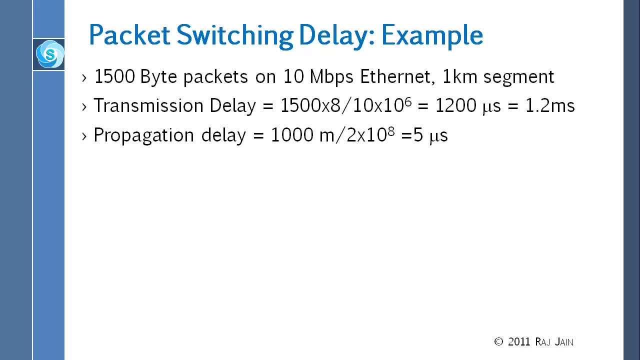 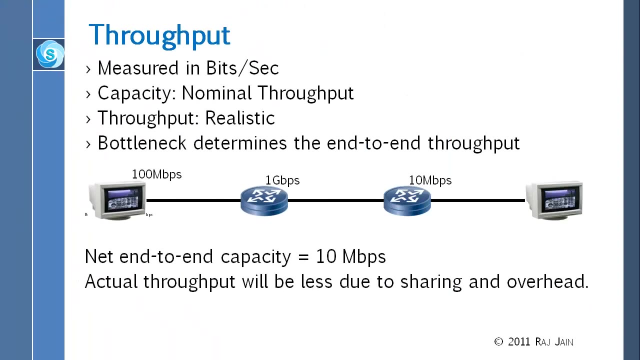 Either 5 microseconds per kilometer for the fiber- the speed of light in fiber- Or if you want to know the speed of light, then 300 meters per microsecond. Either one, Alright. so now we move on to the next measure of performance, and that is throughput. 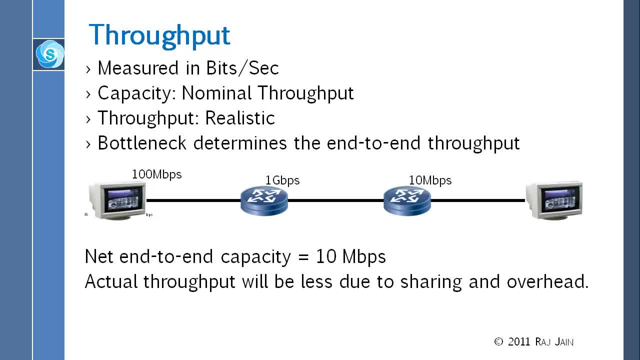 Throughput is measured in bits per second And somebody says capacity, Capacity means nominal throughput, And when we don't say capacity, we mean throughput means realistics. What's the difference? The difference in nominal is what we use in the sales literature. 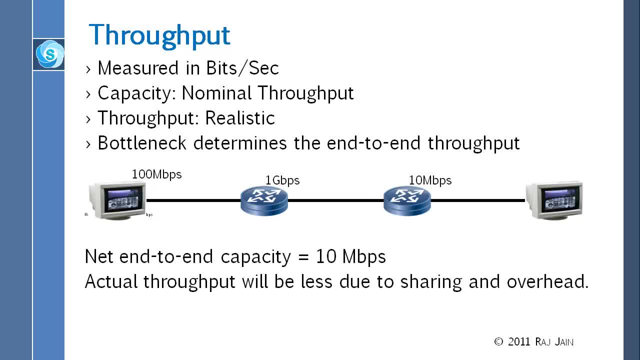 That is the maximum possible. actually, it is not even possible, but that is the rate at which we generally sell. For example, when you buy a Wi-Fi device, They say, let's say it is, Let's say it is 802.11g device. 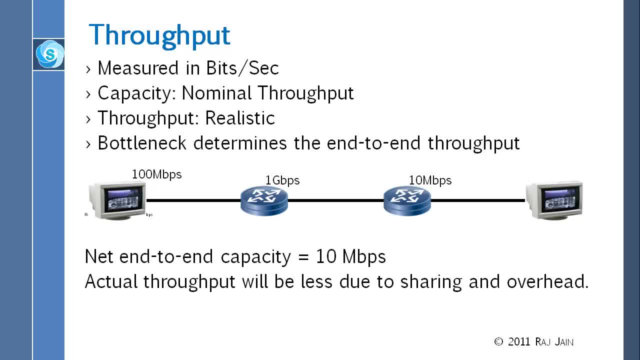 They say it runs at 56 megabits. If you put it on your computer and measure, you will never get any more than 20 megabits. 56 megabits it is sold at, But you will never get any more than 20 megabits. 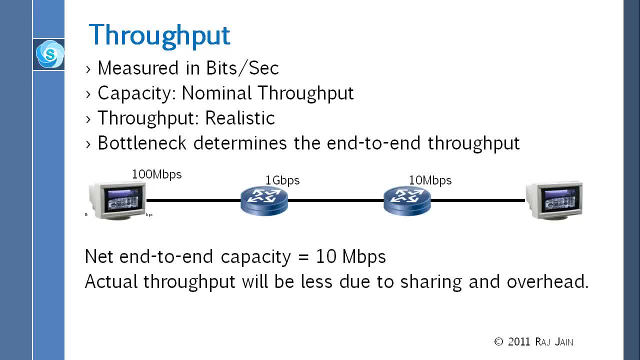 So that 50 megabits per second is actually what is called nominal capacity. That is what each bit. If you were to take one bit on the In the air And measure it, It will be 56 megabits going per second. 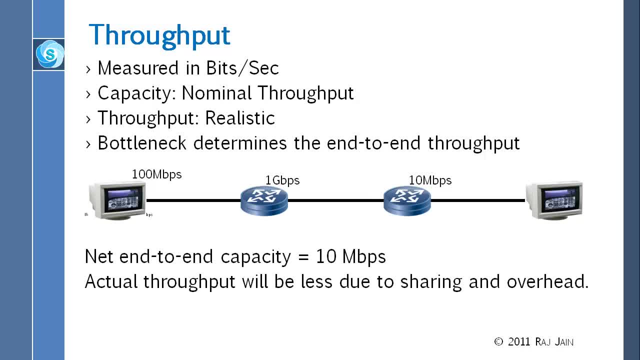 But you are not going to use every bit time there Because a lot of bit time on the wireless You have to wait, You have to collide, You know, And you have to retransmit And so on and so forth. So what you really get in real 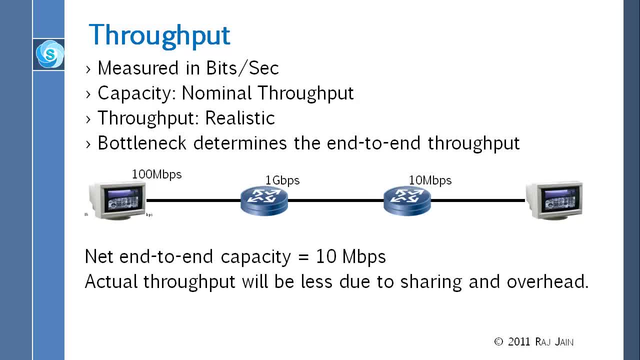 And there is a lot of bits that are lost in the headers. So what you really get as useful throughput is 20.. So your throughput is 20 megabits, But the capacity is 56. So that is a nominal capacity. 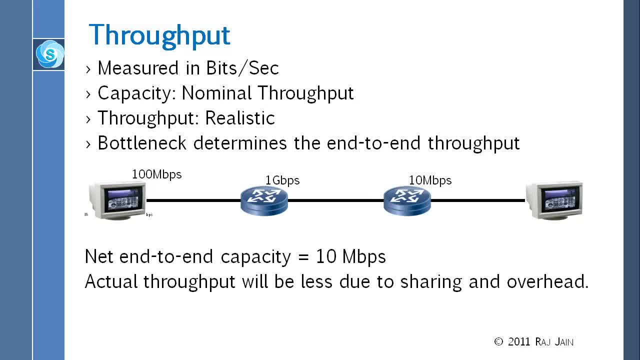 Nominal throughput. Now, if you have many, many links along the path, Your throughput will be determined by the bottleneck. So let's say you have 100 megabits to the first router, Then there is a gigabit between two routers. 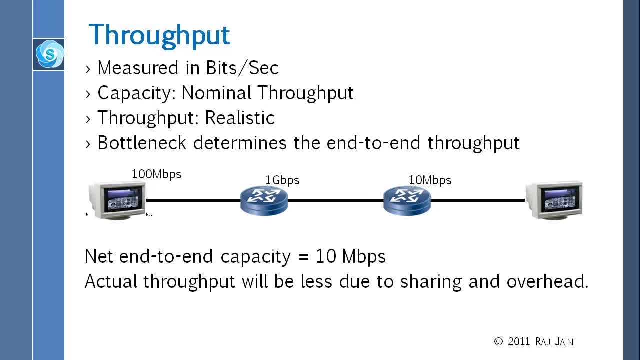 And then 10 megabit to the next computer. What is the speed you will get on this path? 10 megabit, Right. So the end-to-end capacity is only 10 megabit. Actual throughput will be less due to sharing and overhead. 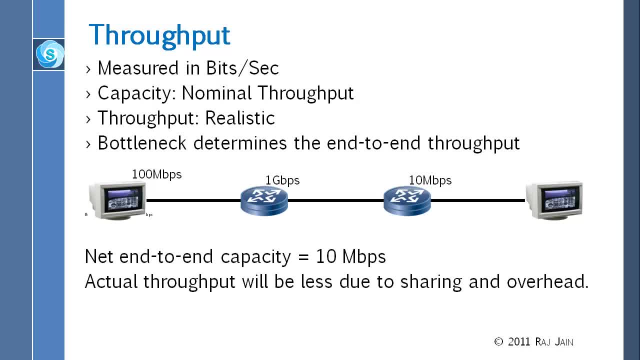 But if suppose you have this connection, If you measure You will not get 10 megabits again, Because again some bits will be lost in the retransmissions And overhead, in the packets And headers And so on and so forth. 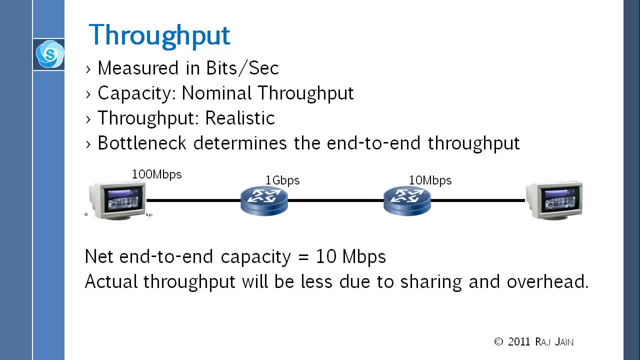 So that is the thing You know. Yeah, So it is still better. Even though the worst Weakest link, The weakest link, is 10 megabits, It is still better than if all three of them are part of 10 megabits. 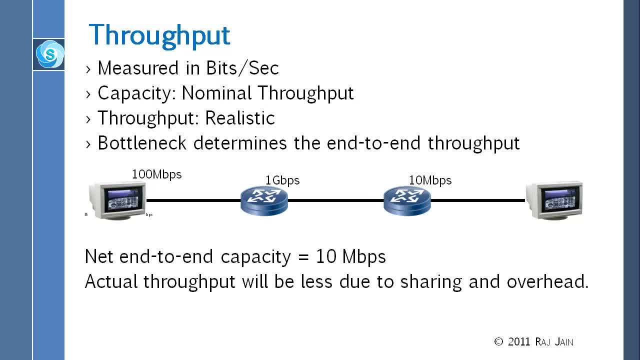 Because part of the journey is still faster. Well, No, Let me just say one more time: The propagation delay does not depend upon the speed, All right. Propagation delay depends upon the distance. Right, This 100 megabit does get the packets on the wire faster from here. 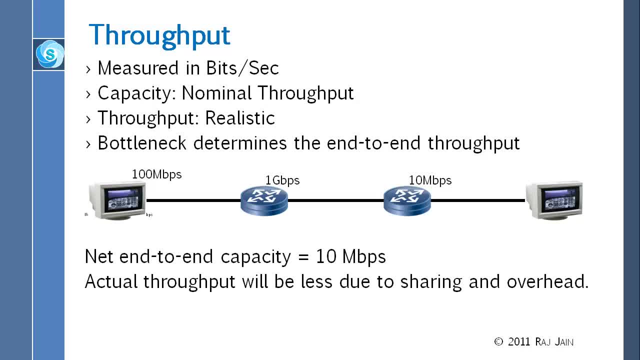 This gigabit does get the packets from this router on the wire faster Here. However, If you don't do things right, It is quite possible that a lot of packets can come in here at gigabits And they are not able to get out. 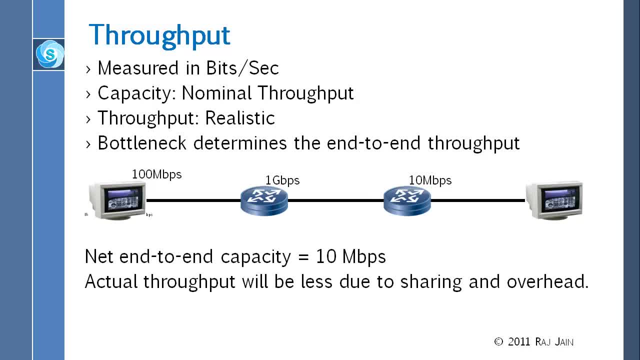 So these queues are very big And the packets start getting lost. Okay, This was the problem 30 years ago When I did my PhD thesis, And that was one of the things that we worked on: Congestion control. What should we do if this happens? 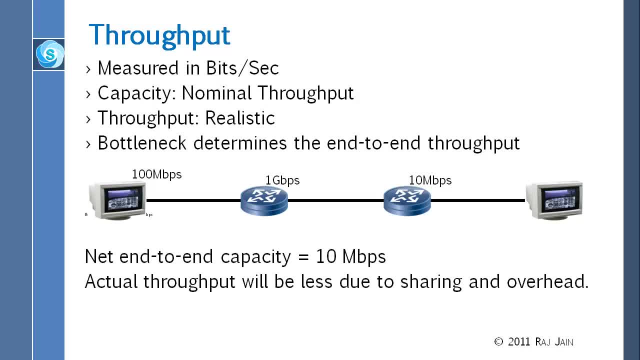 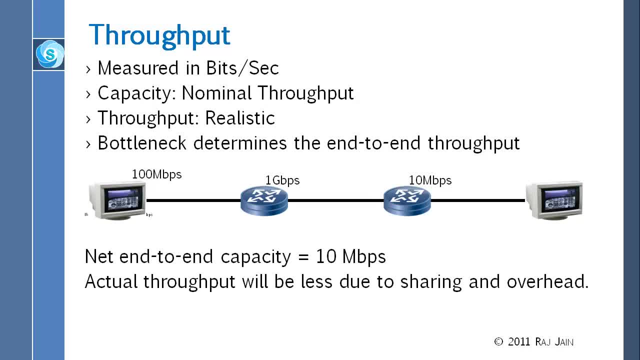 We have a lot of problems. We have a lot of problems. We have a lot of problems, And that was bad. Okay, So you, I mean So your observation is correct That, yeah, If you Given that you want to. 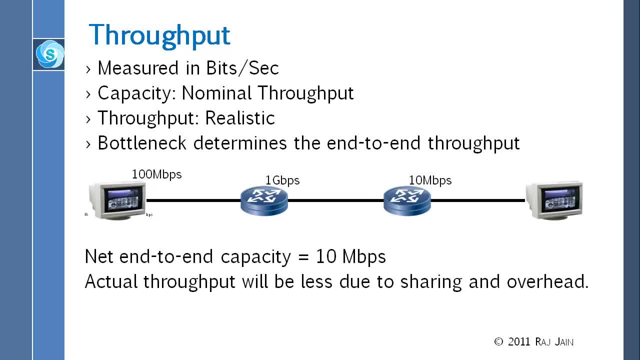 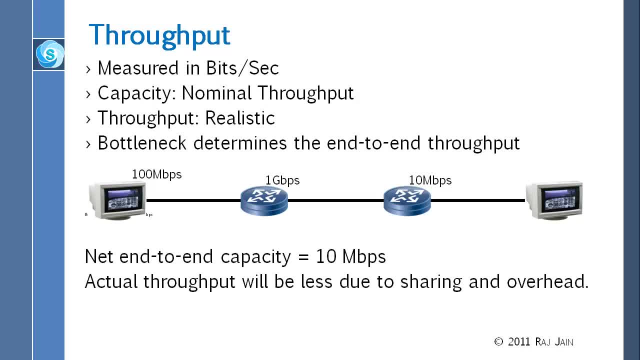 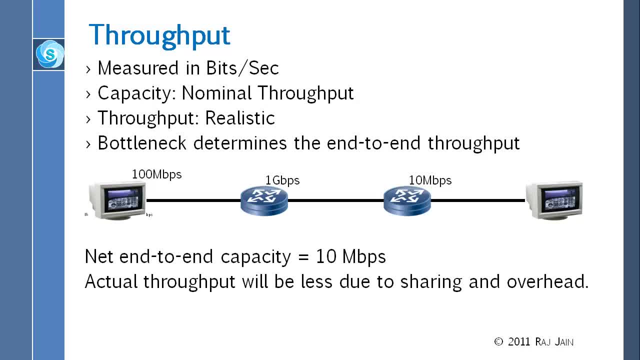 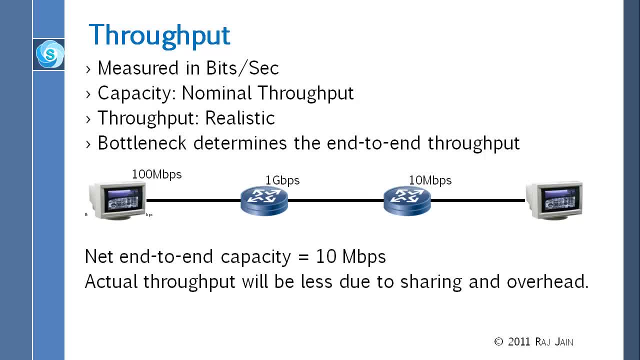 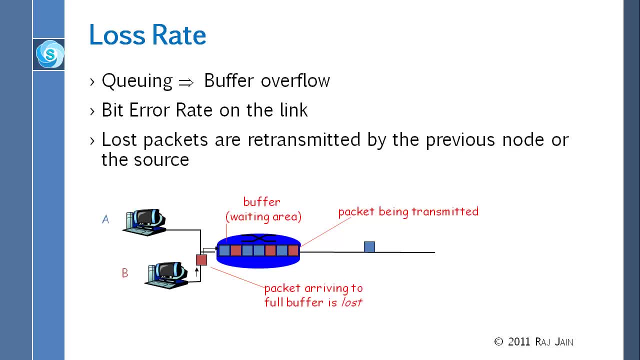 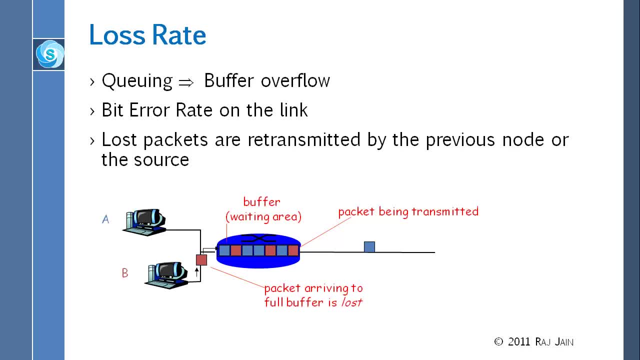 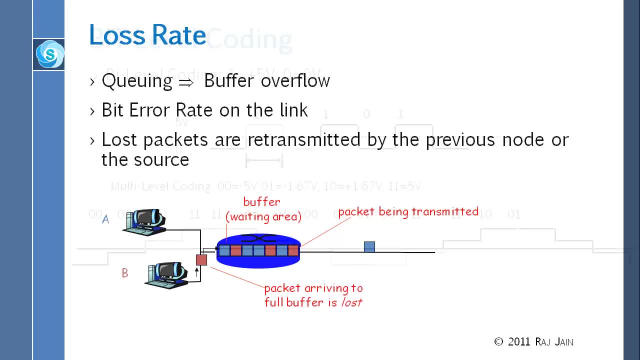 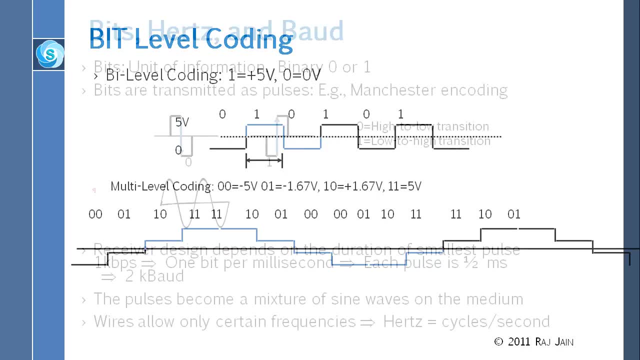 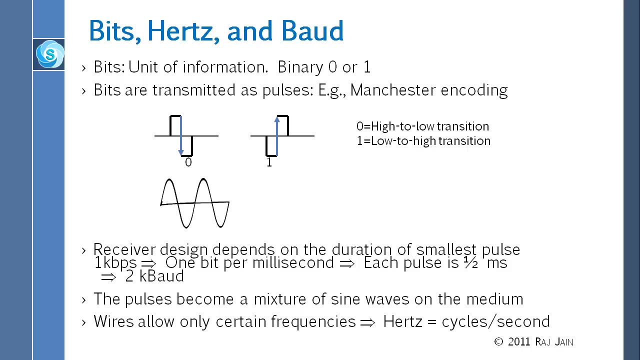 What causes the bit error is that, if you remember this coding thing, if I send these pulses and something like this, right, it is quite possible that, depending upon the distance, this will become smaller and smaller and smaller pulse. At some point the pulse will become so small that the receiver cannot recognize it. 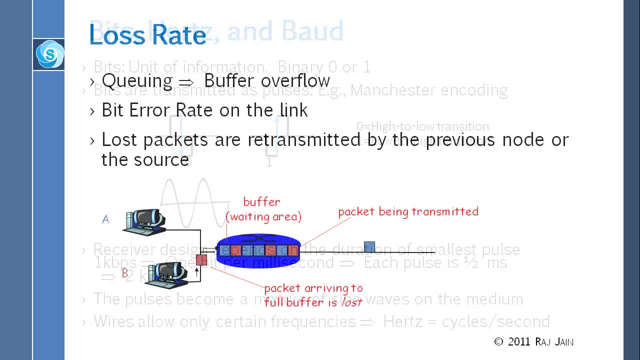 And that will cause the bit error. When you send it on the air wireless, if somebody else sends it at the same time, that will cause the bit error. Any interference will cause the bit error. How could you tell? So we will talk about that when we go to the CRC cyclic redundancy checks. 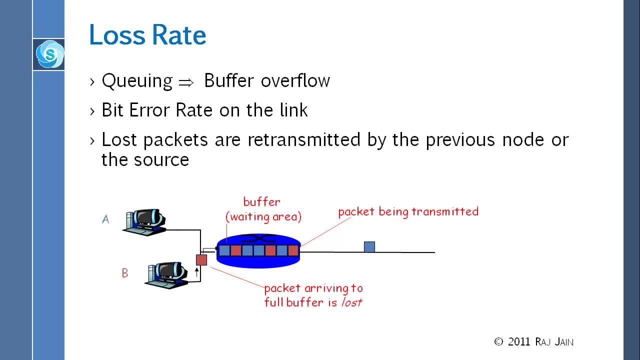 So we put check bits at the end In every packet. If these check bits don't match, then we know that the bit is an error. It's like your credit card number, Credit card number. if you give somebody a credit card number, they don't have to go to the bank. 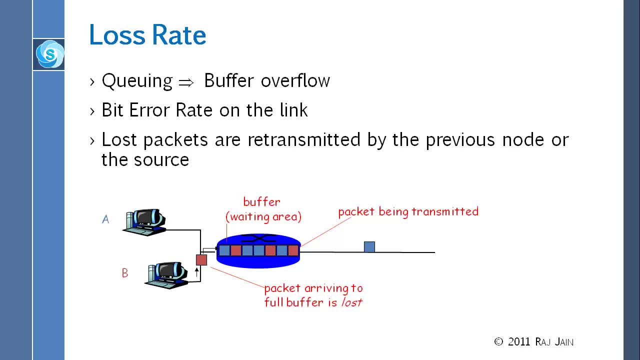 to figure out that this number one digit was wrong, Because there is a check digit at the end, Extra digit. Does the 5 signal get weaker while they are waiting? Okay, so the question is: does the signal get weaker while they are waiting?